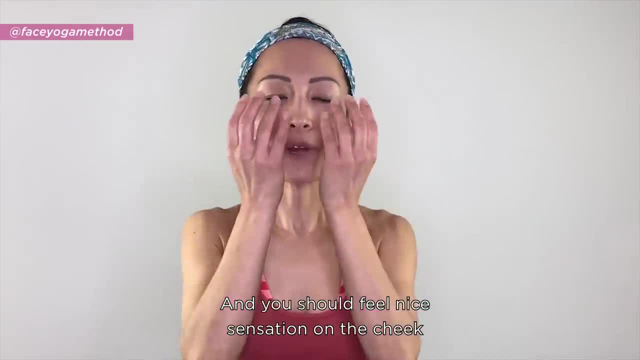 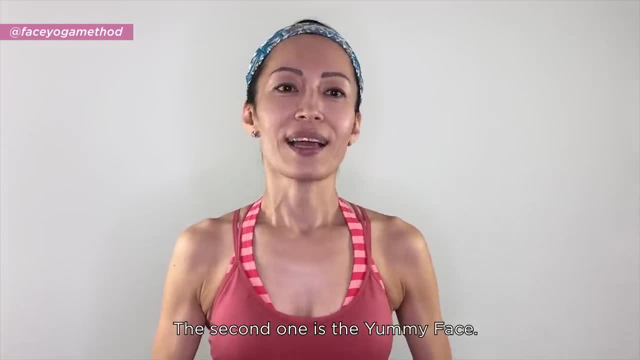 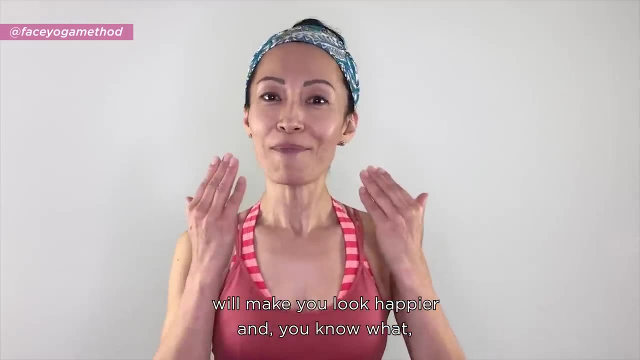 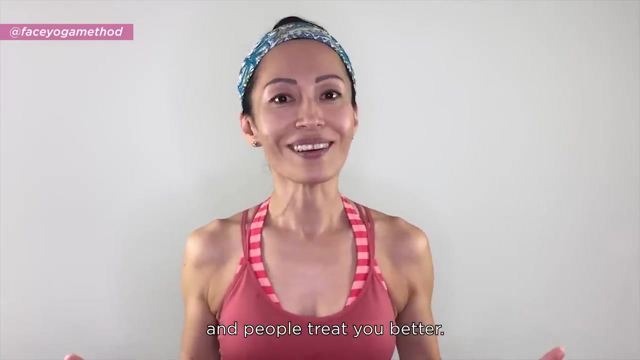 a feeling you want to get right. the second one is your yummy face. i wish i had known this pose, because this pose will make you look happier. and you know what, when you look happy, people around you treat you accordingly and people treat you better. and when you treat it better, you feel. 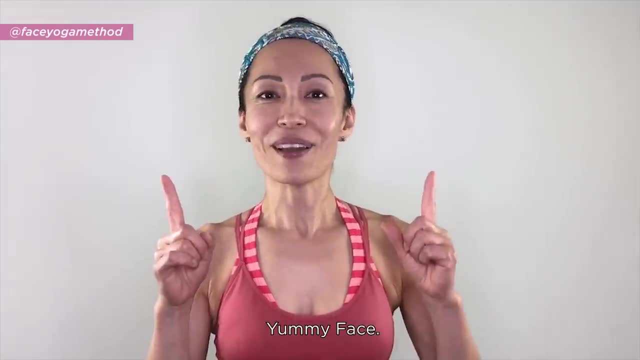 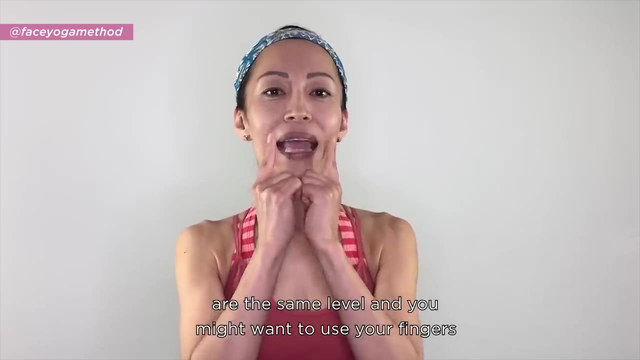 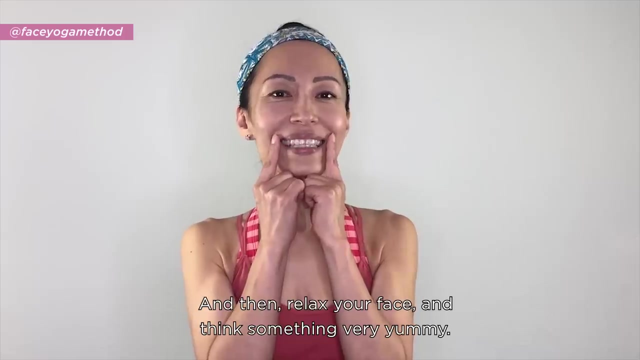 better. it's so worth it to know the pose. yummy face. think about you eating something yummy, yummy and make sure your both corner of the mouth are at the same level, and you might want to use even fingers. just adjust the height and then relax your face and think something very yummy and stick your 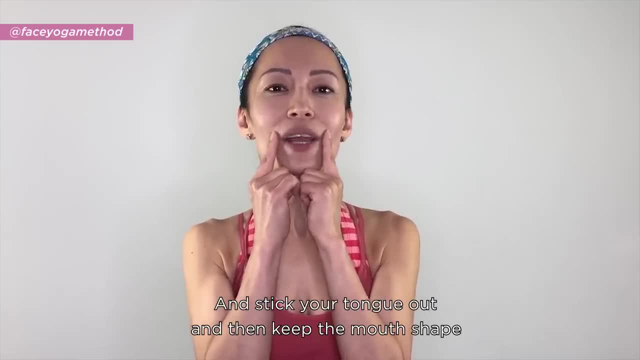 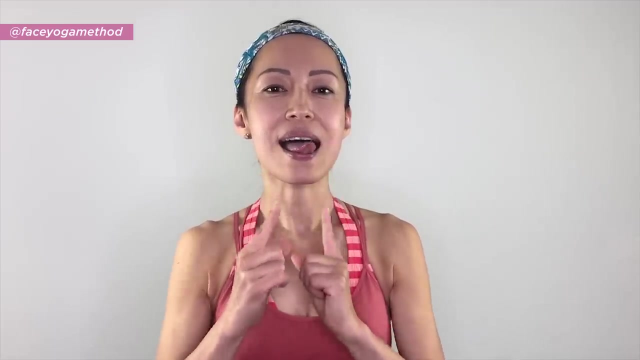 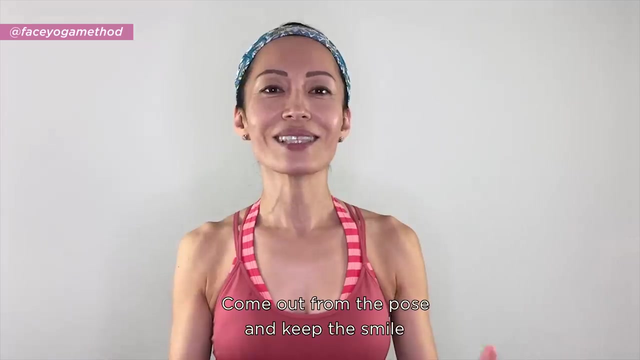 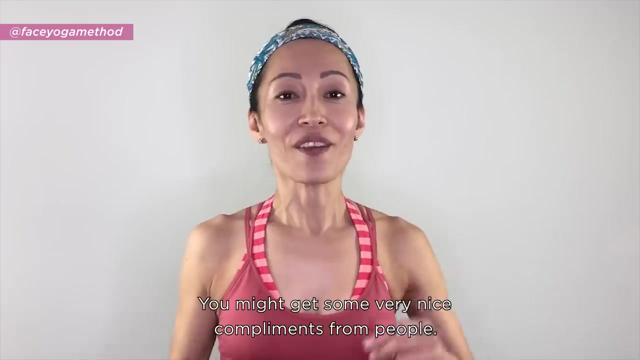 tongue out and then keep the mouth shape and slowly move your tongue left and right to be able to feel the face straight before you bring your hands to the table, come out from the pause and keep this smile throughout the day and see what happens. you might get some very nice compliments from people you never know. and the next one is a. 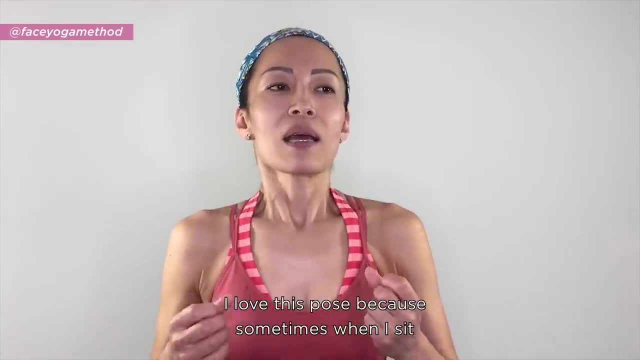 swan neck. oh, i love this pose because sometimes, when i sit in front of computer for a long time, i feel the tightness, my shoulders, i feel the tightness and my shoulders feel tight and i feel my shoulders feel ever much ahead of me. i feel the tightness, my shoulders feel ever much ahead of me. 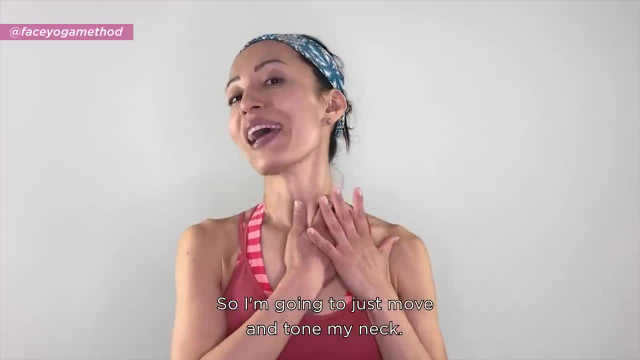 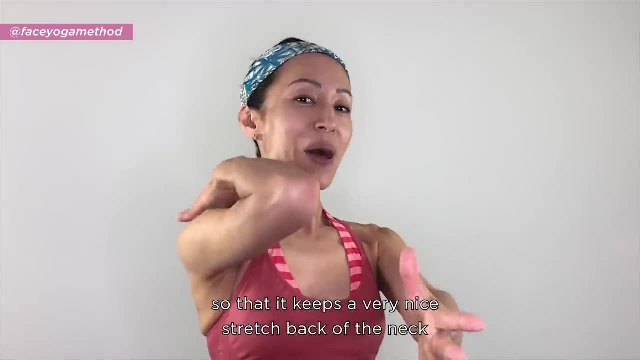 i feel the tightness my shoulders feel ever much ahead of me neck area, So I'm going to just move and toe my neck. So that's one neck, and you want to even add the hand, if you want, so that it gives a really nice stretch back. 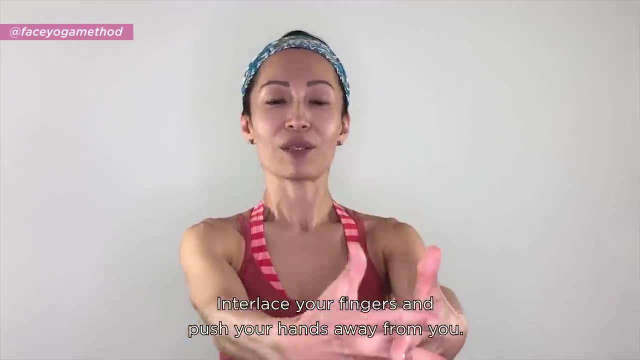 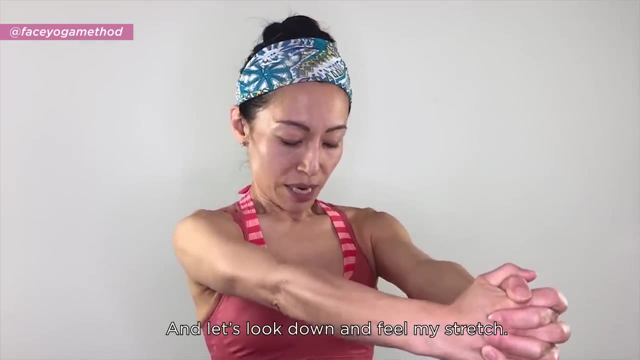 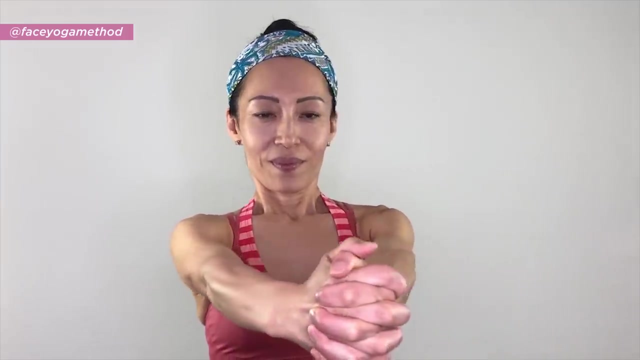 of your neck and between shoulder blades, Interlace your fingers and push your hands away from you And you feel that Good stretch And let's look down a little bit and feel more stretch. I feel it right here And breathe in and out And very. 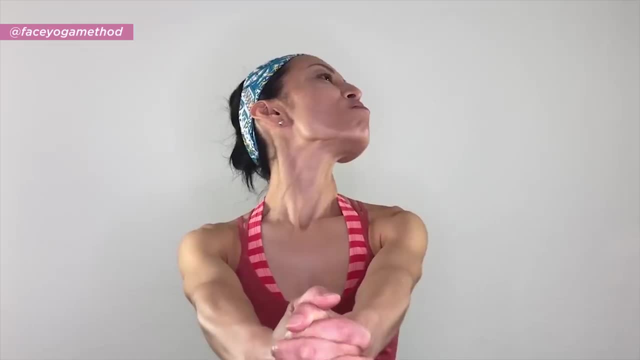 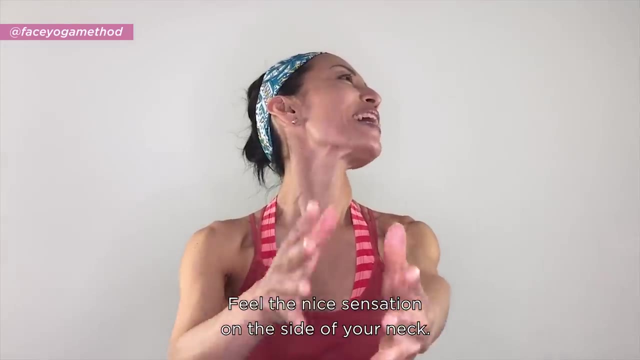 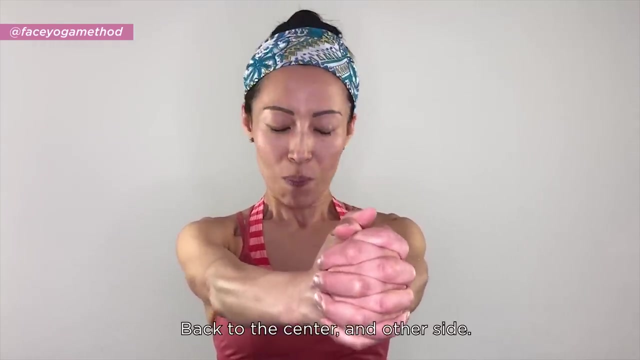 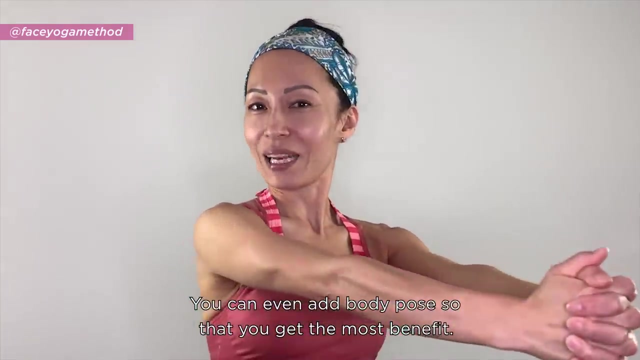 slowly move your chin 45 degree on and back your mouth, Feel the nice sensation on the side of your neck Back to the center and other side back to the center, And you can even add body conserve so that you can get most benefit. Let's do it. So move your hands to one. 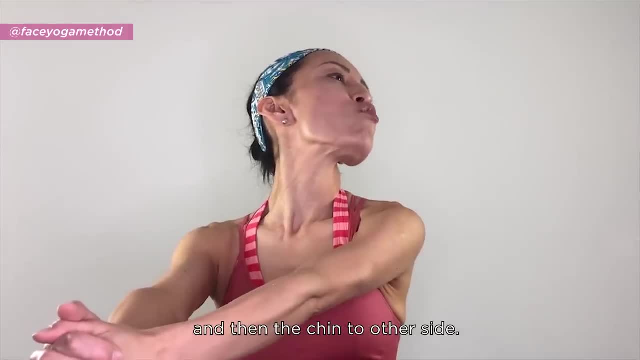 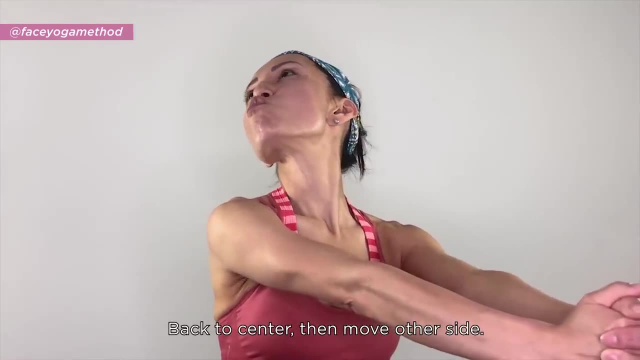 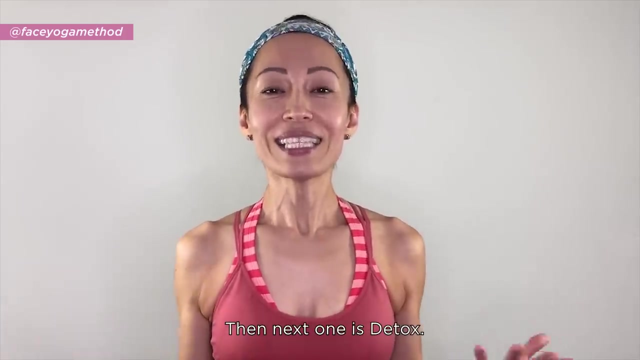 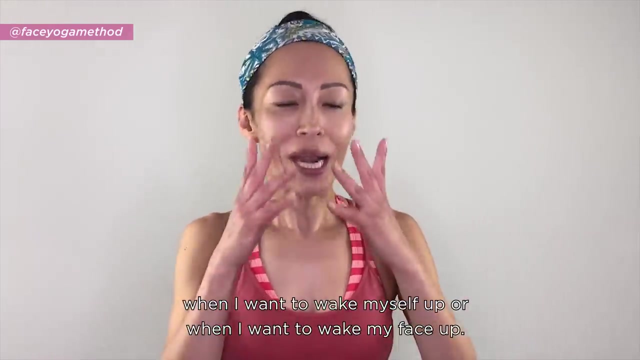 side and then your chin to other side. Ooh, I feel it. Relax your forehead Back to center and other side. Shake it out. The next one is detox, This one. I love to do this in the morning when I want to wake myself up, or when I want to wake my face up, or when I get a little bit. 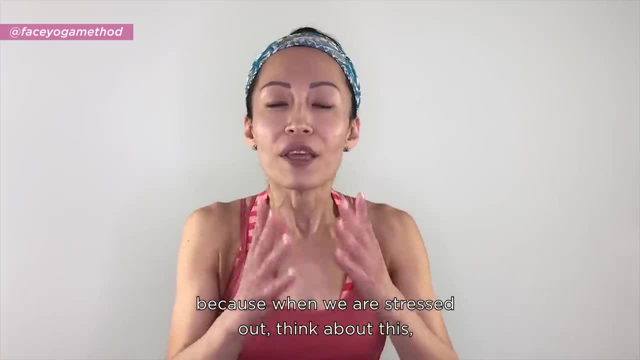 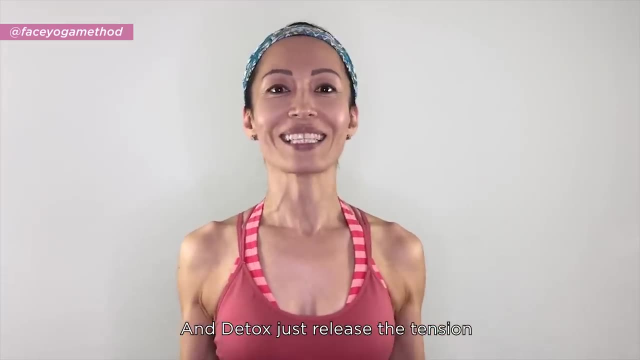 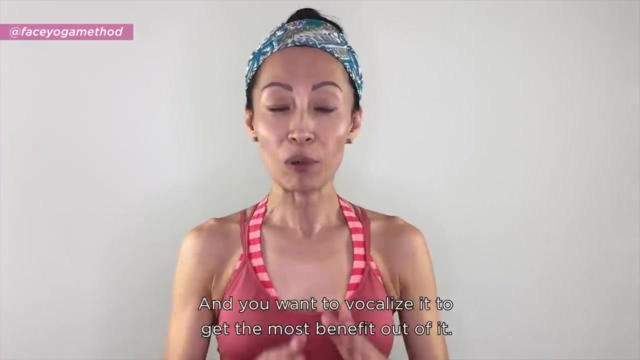 stressed out. I do this because when we are stressed out, think about this. We hold our breath, We tighten our body and detox. Just release the tension and you can even add hands or like this or this. So breathe in, Pretty simple and you want to vocalize it to get the 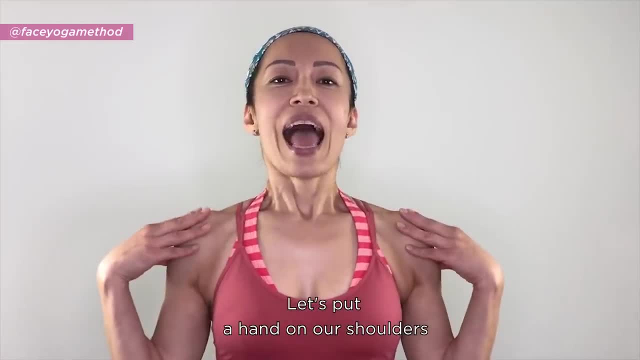 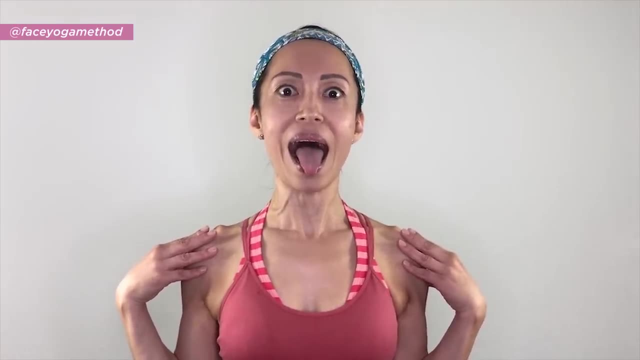 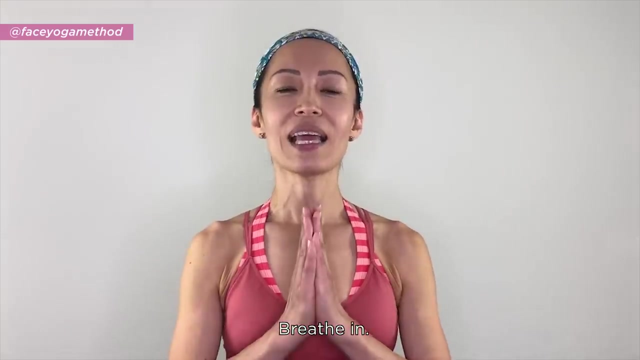 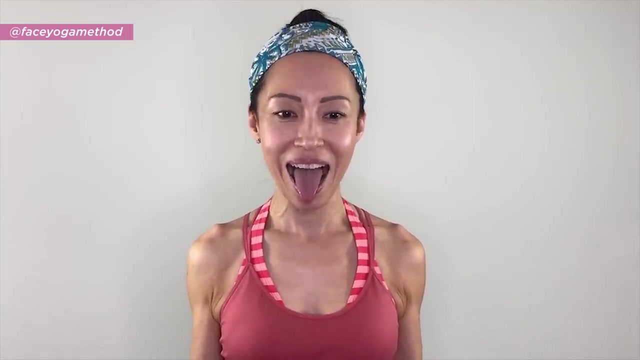 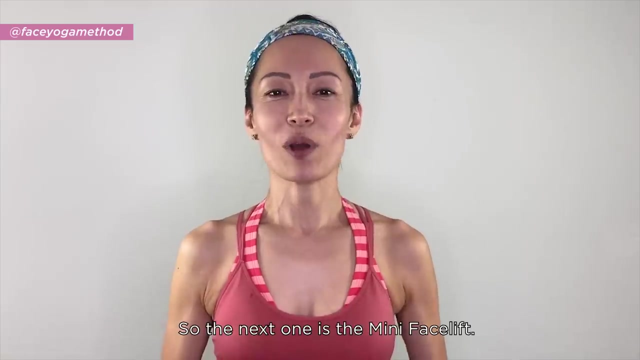 most benefit out of it. Let's put a hand on our shoulders and relax the forehead, and then, ah, Come up from the pose. Let's add this hand movement: Breathe in, Breathe out. Did you feel that? I felt it? So the next one is the mini facelift. Just really lift up your face. 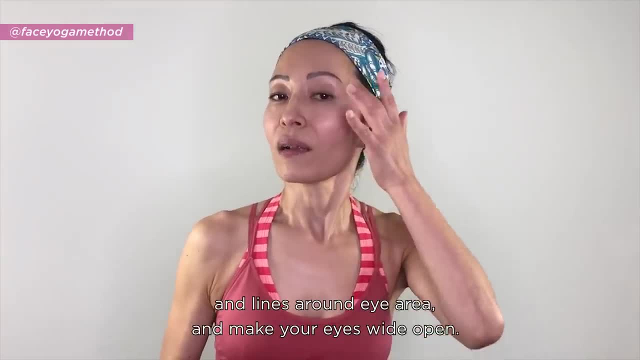 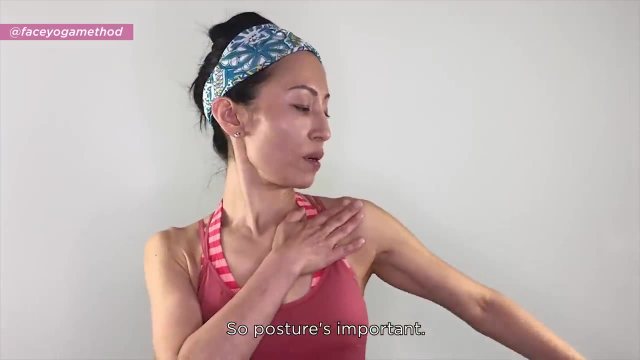 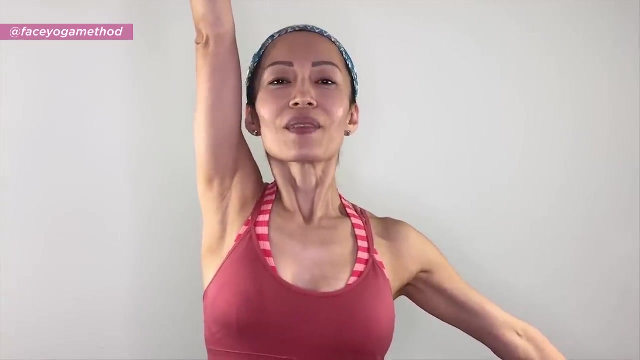 Get rid of all the nasolabial lines and all the muscles Lines around eye area and make your eyes wide open. So posture is important. Forty-five degree, angle Your arm and other side up, Breathe in and out from your nose and without. 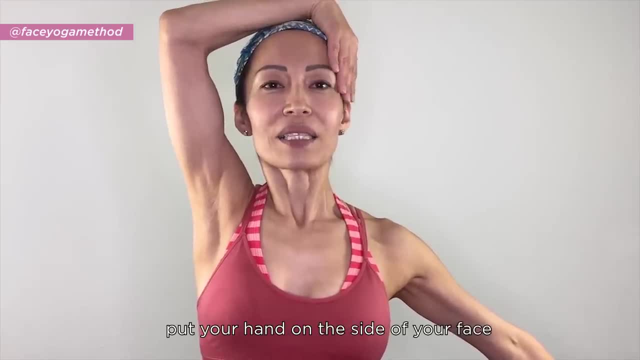 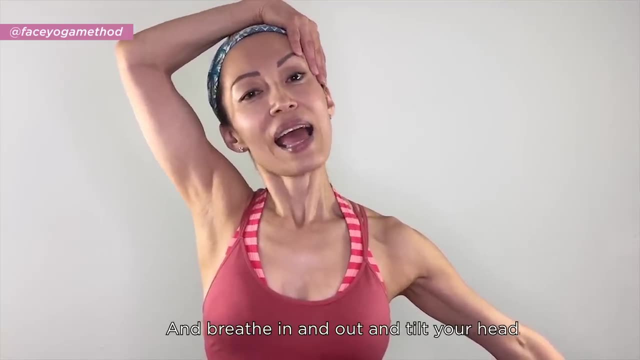 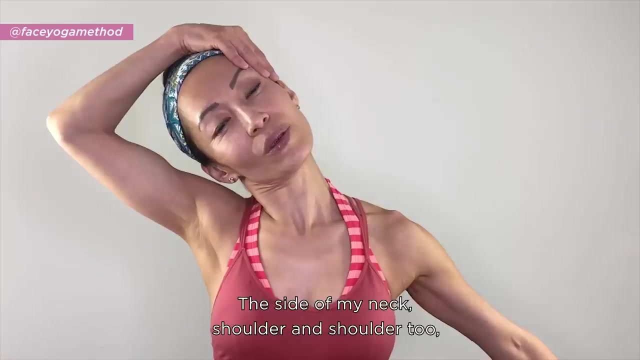 tilting your head. put your hand on the side of your face and pull forty-five degree angle, Very slight, And breathe in and out and tilt your head And woo, woo, woo, I feel good. Stretch the side of my neck, shoulder and shoulder to my fingertips.